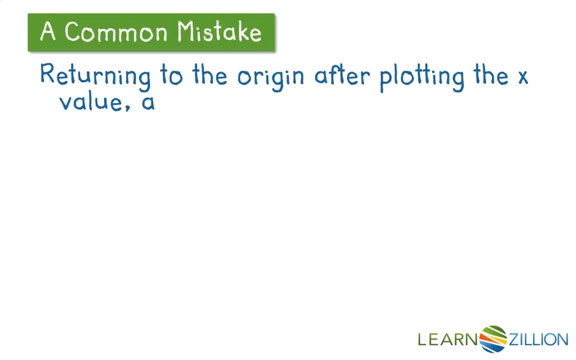 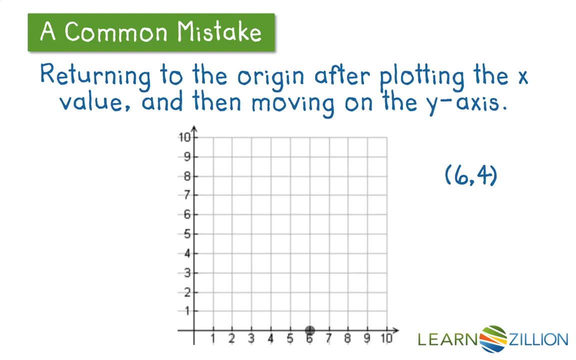 Another common mistake that I've seen people make is that they return to the origin after plotting the x-value and then they move on the y-axis. So if the ordered pair was six- four, they would plot a point at six and then go back to the origin and plot a point at four. 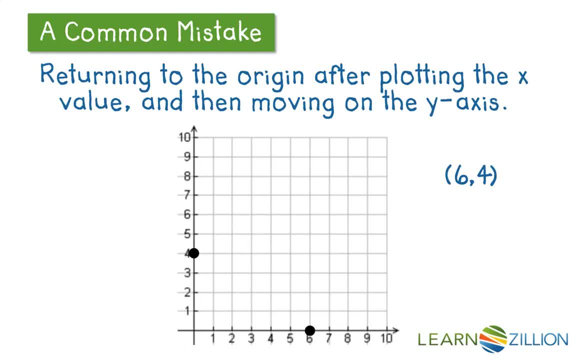 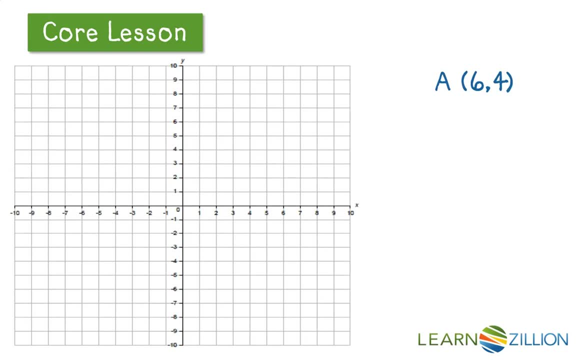 Now the ordered pair of six- four is just one point on the coordinate plane. Alright, let's start by plotting this first point A on the coordinate plane. A has a positive six and a positive four. It's going to put it in quadrant one. 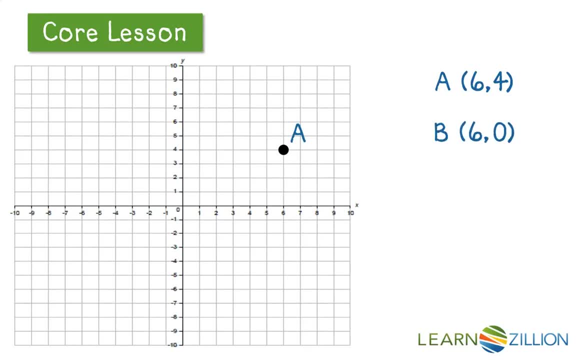 At point A: six four. Let's try point B at six zero. Now it has a positive x-value of six, but it has a zero value for the y-value And so it doesn't move anywhere. It stays right there on the x-axis. 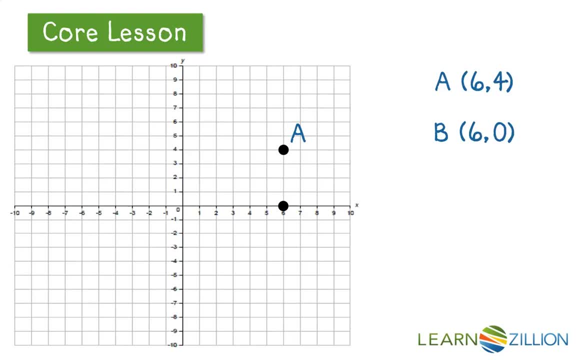 Now the question for today is: what's the distance between these two points? Now we could count the distance as units from one point to the other, Kind of like this: I could just start counting One, two, three, four units And I can see that the distance is one point. 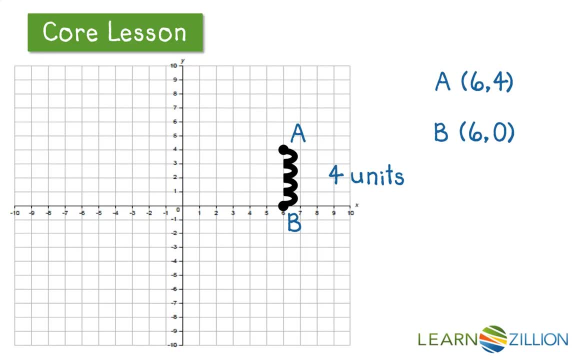 And I can see that the distance is four units. But you know, there's a much more effective way, And this is using absolute value. Alright, in order for us to find the absolute value, the first thing we do is we notice that. hey, guess what? 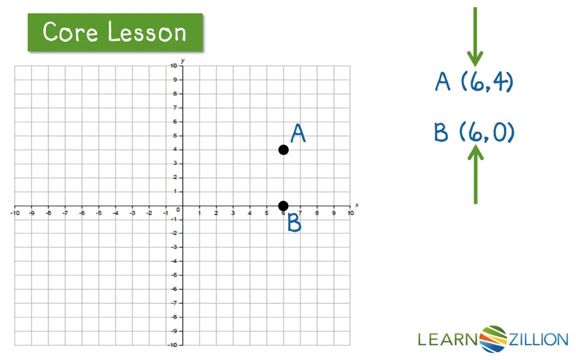 both of these ordered pairs have the same x-value. Now, because they have the same x-value, we're going to find the distance between the y-values. Now we want to find the difference between the four and the zero. This difference is going to give us the length between the two points. 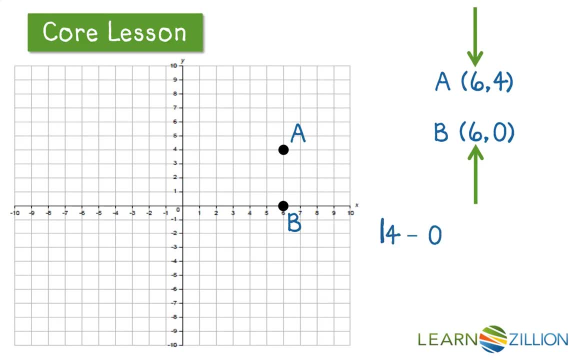 Now there are two ways I can find this. I can find the absolute value of four minus zero, which equals the absolute value of four, which equals four, Telling me that the distance between points A and B is four. Or I could try it starting with the B. 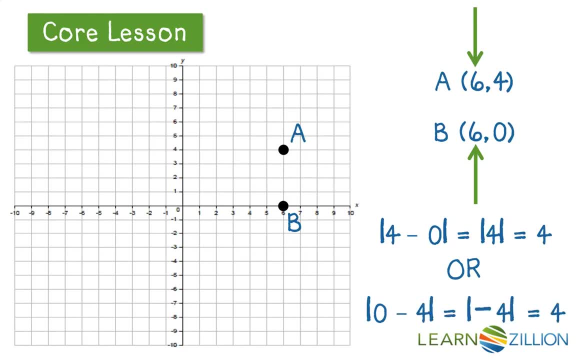 I could start with zero And I could do. the absolute value of zero minus four Gives me an absolute value of negative four, Which, guess what, since we're talking about distance, it's always positive. It's four units. So you can see that I've used absolute value.